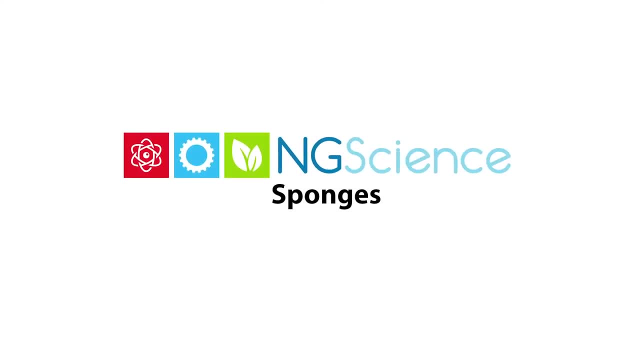 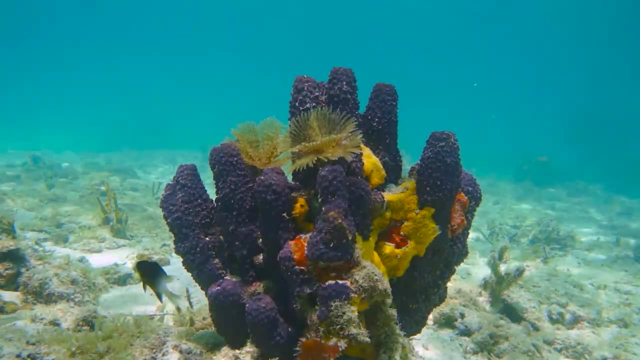 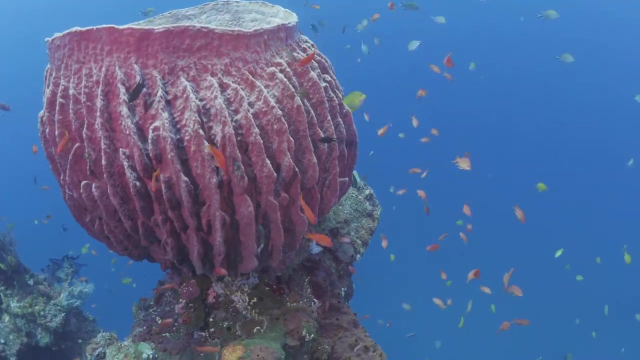 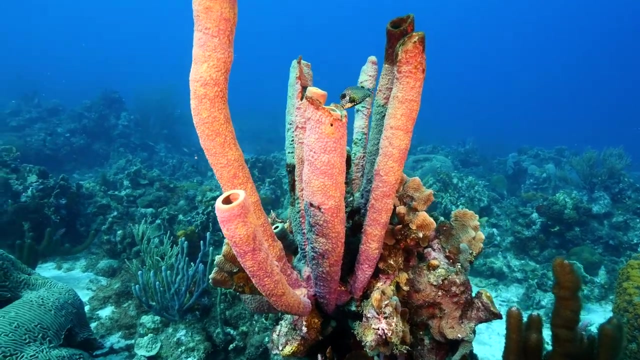 Sponges are some of the world's oldest and simplest animals. They are multicellular organisms but do not have body parts, tissues or organs. Their asymmetrical bodies consist of one or more tubes with an opening at the top. An asymmetrical body does not have any lines of symmetry. 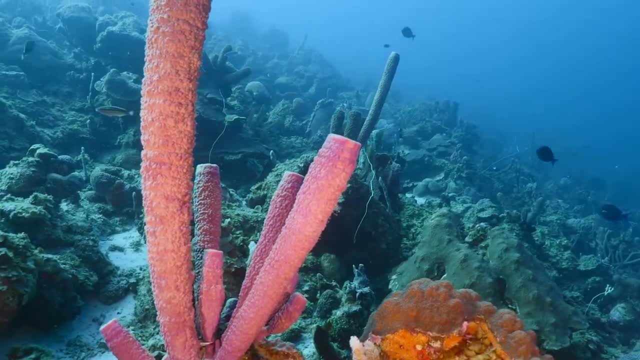 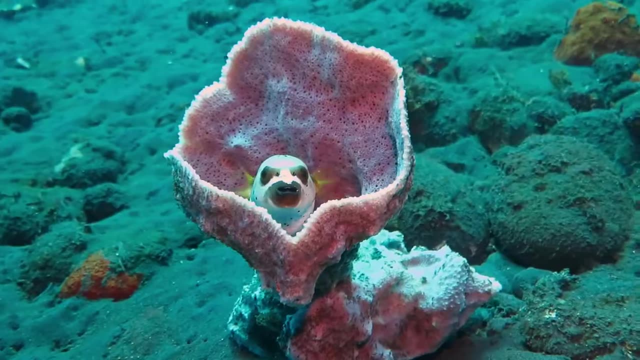 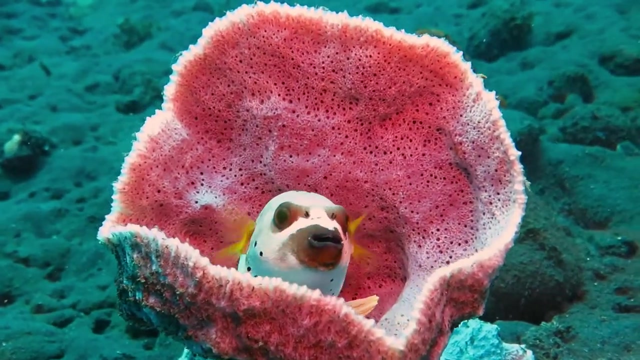 Most sponges live in the ocean, but some live in freshwater environments. Sponges are filter feeders. They pump seawater through the holes in their body called pores. As water moves through the pores, bacteria and tiny particles are taken up from the water. as 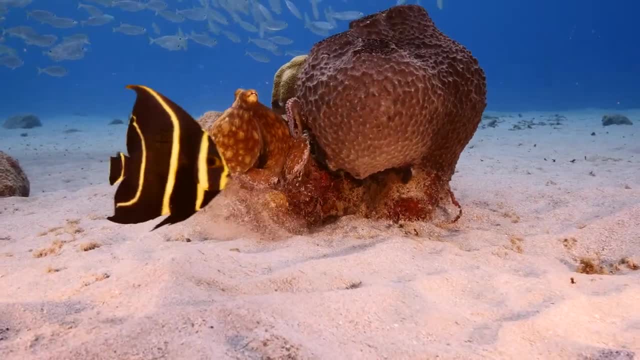 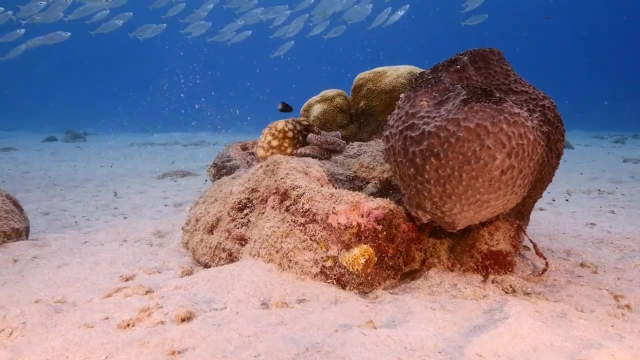 food. Sponges do not move about and rely on a continual flow of water through their bodies to evolve. They are not able to move around. They are not able to move around. They are not able to obtain food, oxygen and remove wastes. Sponges usually reproduce sexually, but some 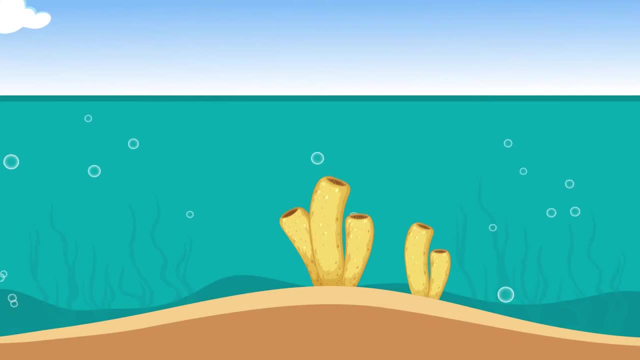 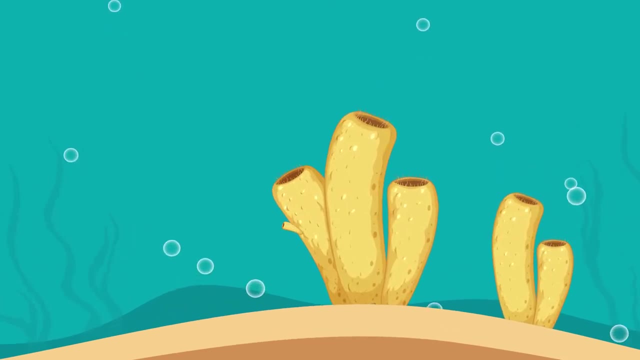 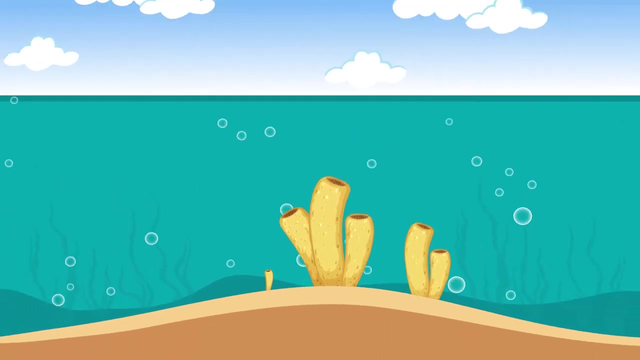 reproduce asexually by budding. Budding is the process in which a new organism develops from an outgrowth on the body of a parent organism. Once developed, the offspring detaches as a new organism that is genetically identical to its parent. Hey, Want to know something really. 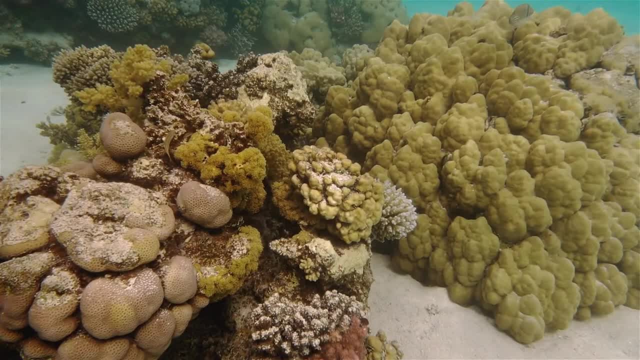 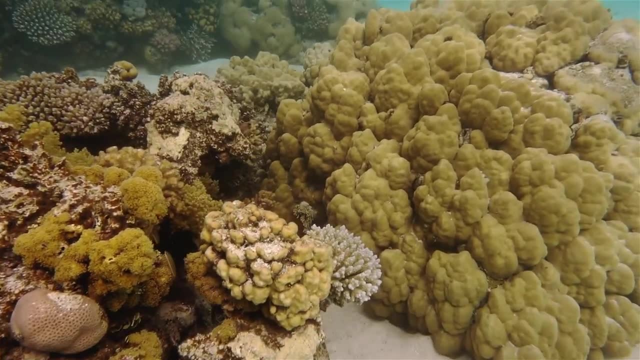 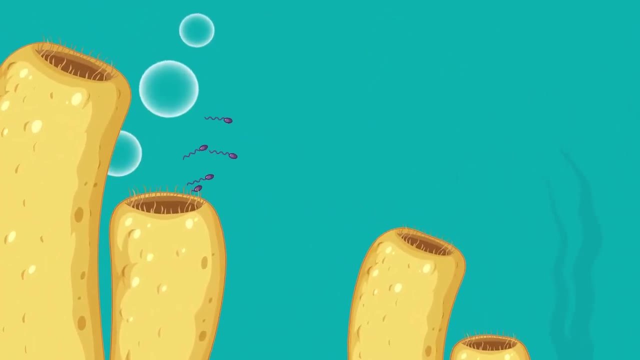 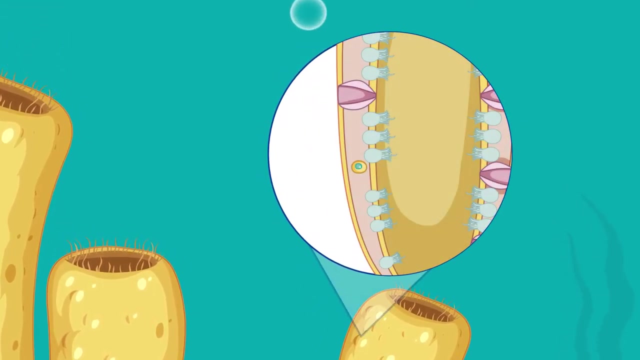 interesting about sponges. Let us know in the comments below. They're hermaphrodites. This means they can function as both sexes- male and female- simultaneously. During sexual reproduction, male sperm cells are released into the water. The sperm cells enter other sponges and fertilise female egg cells. 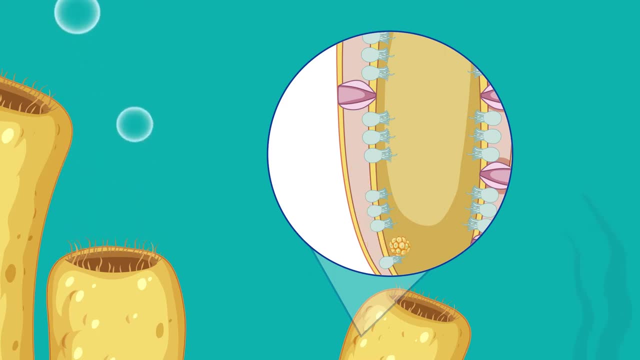 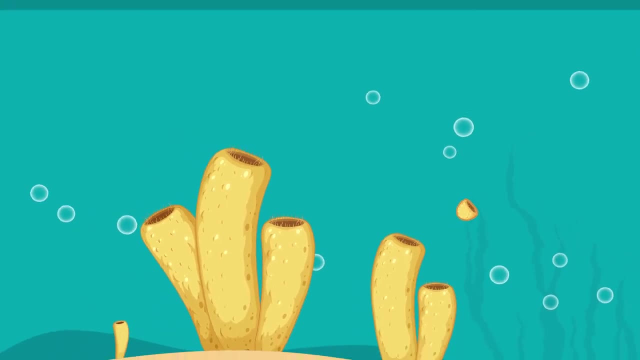 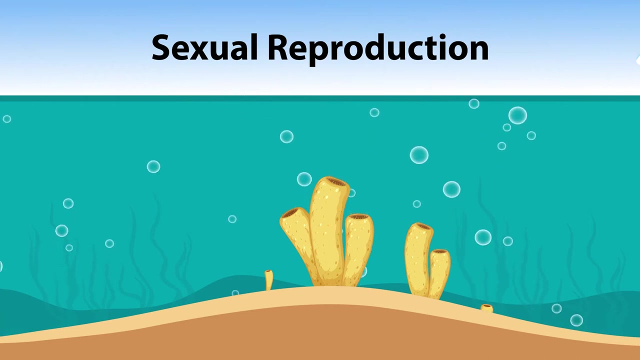 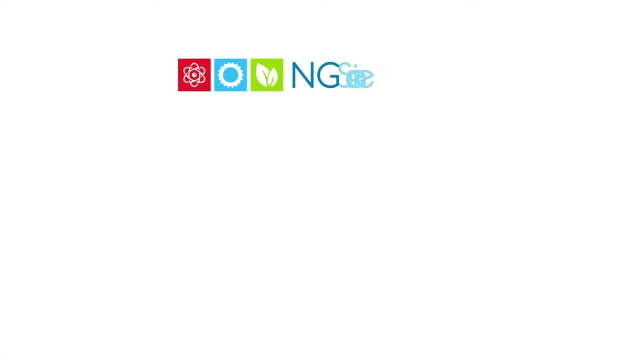 The egg cells develop into free-swimming larvae and are released into the water. The larvae eventually find a place to settle and attach themselves to the sea floor, And the life cycle of these strange and simple animals continues. Don't forget to subscribe.